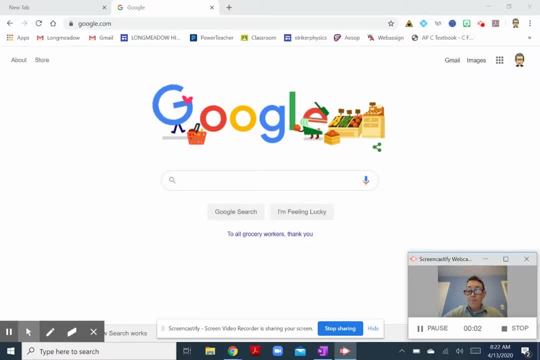 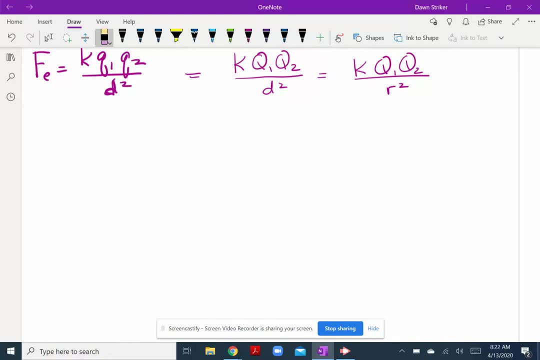 Hi folks, I'm going to try to record one more example problem using Coulomb's Law, but solving for something different this time. Last time we were solving for the electrostatic force between two charges, and now I'd like to solve for the distance between two charges. If 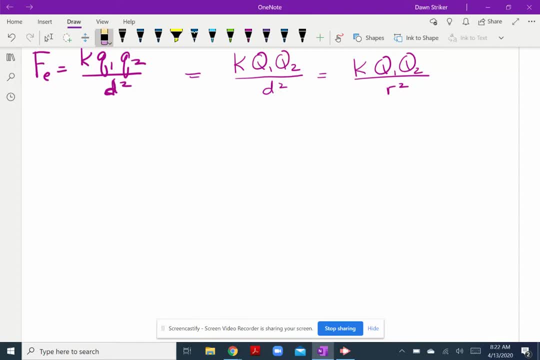 we're given the force and we're given the size of the charges, could we solve for the distance? All right, So a different application of Coulomb's Law. I'm going to try to get my head out of this picture. No, maybe I'm not going to do that, but I am going to tilt this down. 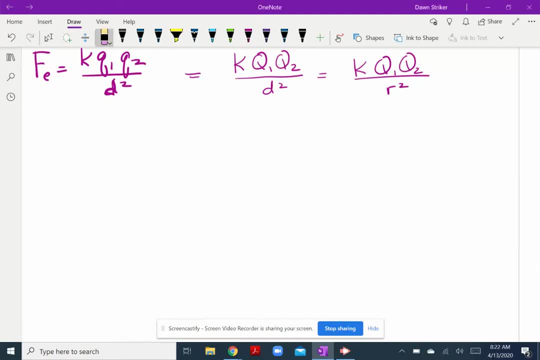 so that I can draw on my tablet. Okay, So let's do the example of two charges where I know the size of the charges, I know how much charge there is And I know the force that's experienced. So let's say this charge, maybe it's a metal conductor. 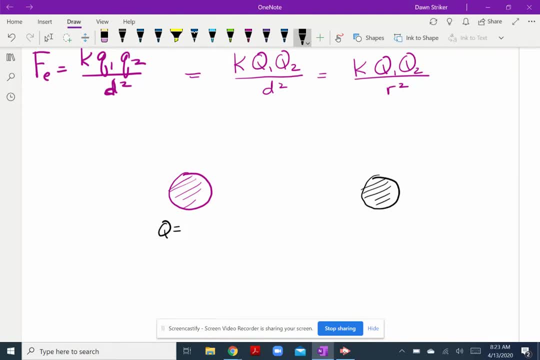 that has some extra electrons on it And let's say the charge is, I don't know- five times 10 to the negative six Coulombs. So that means it's lost some electrons because it's got a positive charge. And let's say this Q2 has also lost some of its electrons. 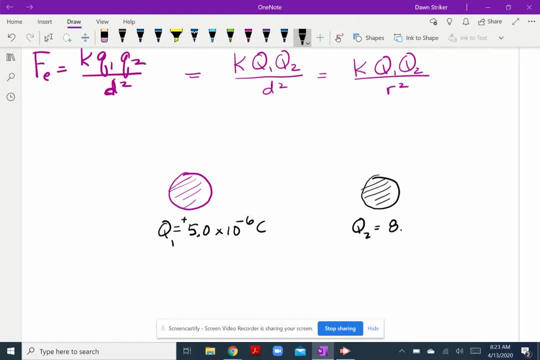 And it's got a positive charge of how? about eight times 10 to the negative six Coulombs And if they've both lost some electrons, so that they're both positively charged. I know that the force is going to be pointing away, And so now we have to choose a size of. 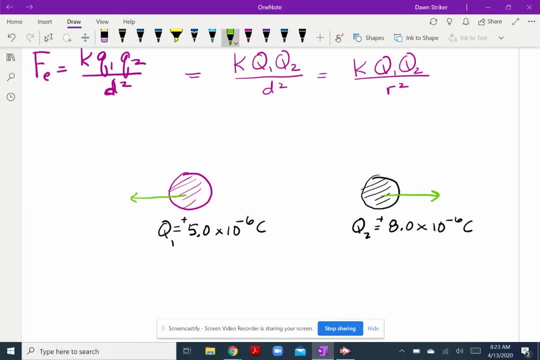 the force. So what do you think? How about a quarter of a Newton? So Fe is equal to 0.25 Newton, Electrostatic force is equal to 0.25 Newton. So, given the charges and given the size of the force, can I find the distance between them? D? 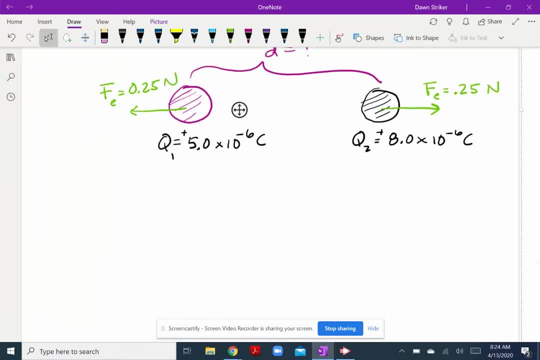 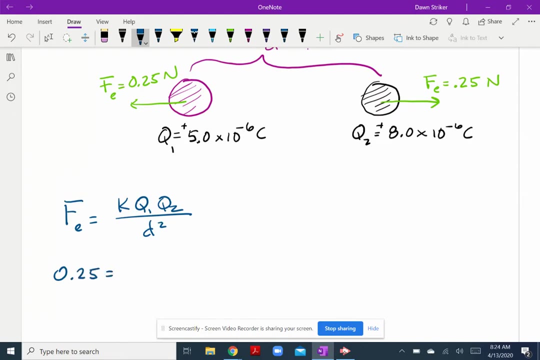 Can I find that distance? And so that's what I'd like to do. All right, So I'm going to use my Coulombs law. Fe is equal to KQ1Q2 over D squared. I'm just going to plug in everything that I have and solve. So 0.25 is equal to nine times 10 to the nine. 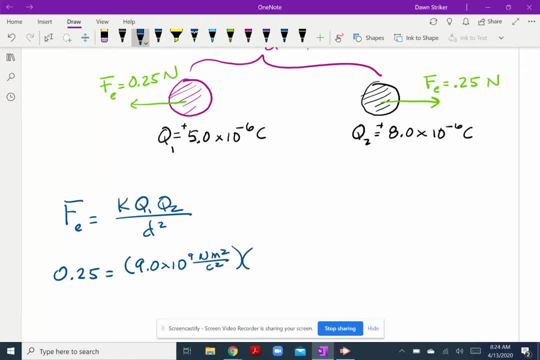 Newton meters squared per Coulombs squared, One of the charges five times 10 to the negative six Coulombs. The other one is eight times 10 to the negative six Coulombs. And, last but not least, divide by D squared, which is the thing I don't know. 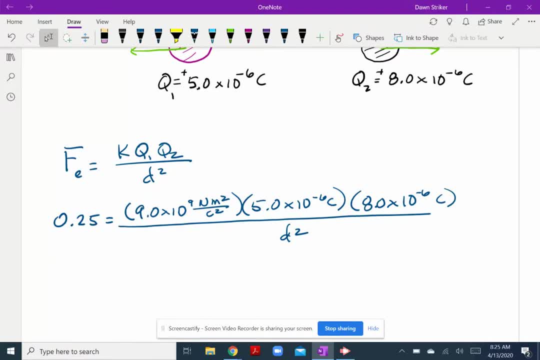 So I can solve. I can multiply these three numbers on the top first, 0.25.. That's, a Newton is equal to. But before I do that, let's pay attention to the units. And so I've got Newton meters per meter. 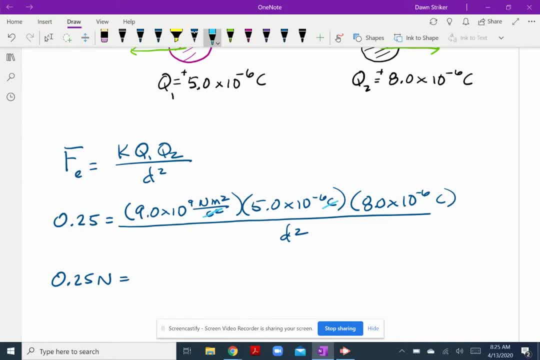 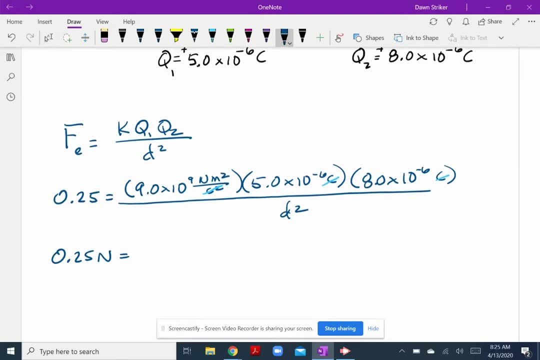 squared on the top And then on the bottom, I've got a Coulombs squared but Coulombs squared, and Coulombs and Coulombs will cancel, And so that's going to leave me with a Newton meter squared on the top, And so nine times 10 to the nine, using my calculator, you could calculate with me, because 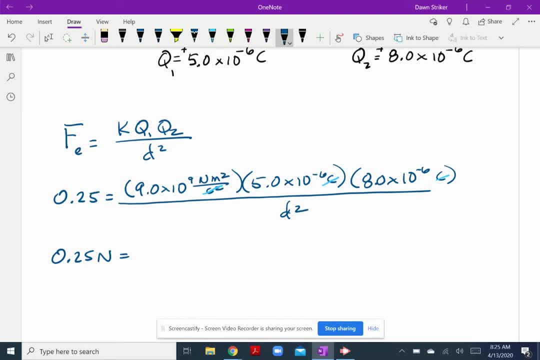 sometimes I make mistakes. Nine times 10 to the nine times five times 10 to the negative, six times eight times 10 to the negative six, And I get 0.36.. So 0.36. And again, that is a. 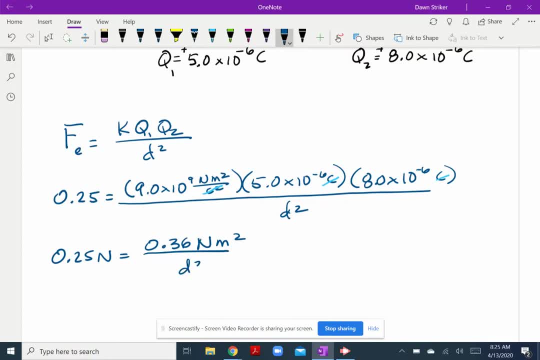 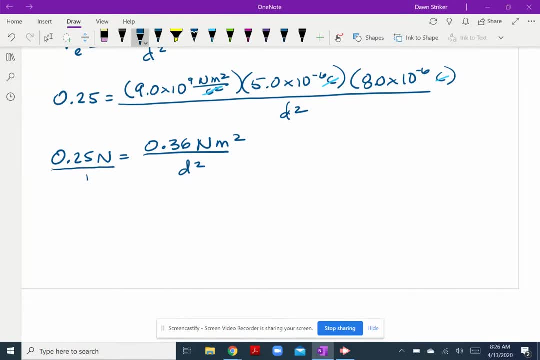 Newton meters squared over D squared. So there I am. So now, what do I do? Well, this 0.25 Newtons is really the same as 0.25 divided by one. you think about it that way. you could cross, multiply. So 0.25 newtons divided by 1 is equal. 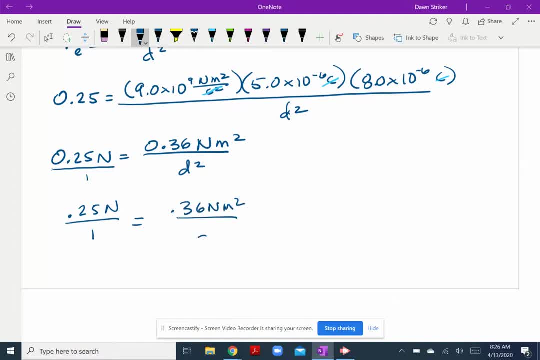 to 0.36 newton meters squared divided by d squared Cross, multiplying, multiply those and then multiply those, And what you'd like to do is solve for d squared, And so if you do that you get 0.25 newtons times d squared is equal to 1 times 0.36.. So 0.36 newton meters squared. 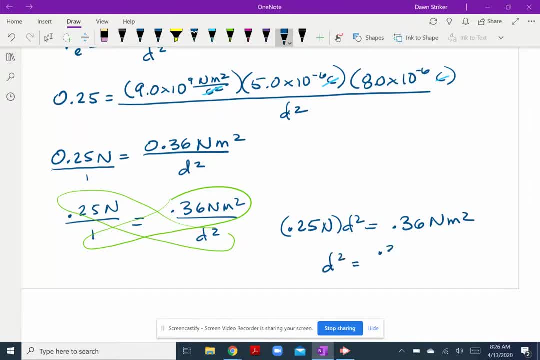 So then I can see that d squared is going to be equal to 0.36 newton meters squared divided by 0.25 newtons. And look at those units. I love it when the units work out that way. Okay, so I'm going to get a number that has a unit of a meter squared.